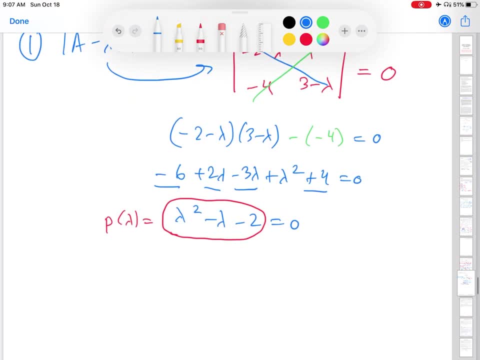 So my job now is to solve this for lambda, to find the roots of this polynomial. There are lots of things I could do. This is a quadratic equation. I could use a quadratic formula or I could try to factor Right. So that would be my first suggestion: to try. 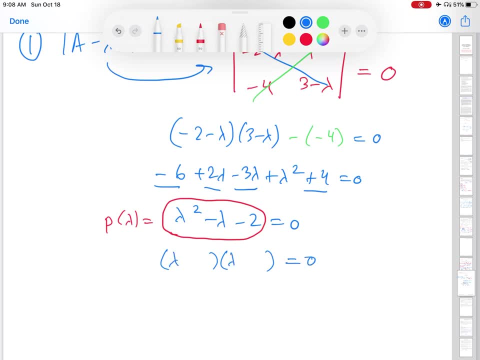 So if I try to factor then it looks like lambda plus 2, lambda minus 1 is going to work. So is that true? No, it does not. I have to switch the signs here, So I have to do lambda minus 2, lambda plus 1.. So it's a quick check: Lambda squared plus lambda minus 2, lambda gets me that negative, And then negative 2 times 1 gets me that minus 2.. All right, So that works out. So now that I have factored it, I can find my lambda values. So I get lambda equals negative 1 and lambda equals 2.. Great, So I have found the eigenvalues. These are the e values. 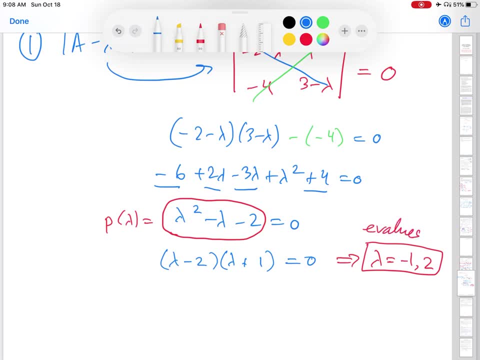 How do I find the eigenvectors? Well, I'm going to go back to an intermediate step in the previous video. Right, Remember that before we got to this condition, we got to this condition by taking a v equals lambda v, the definition of what it means for v and lambda to be eigenvector and eigenvalues respectively, And we had expressed the equation. 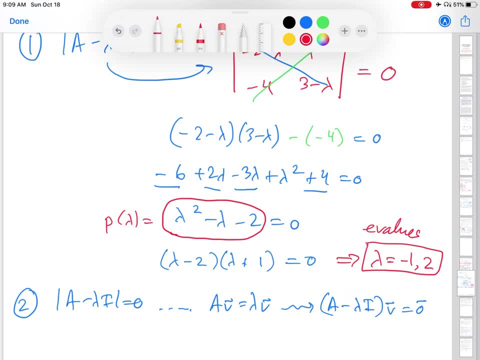 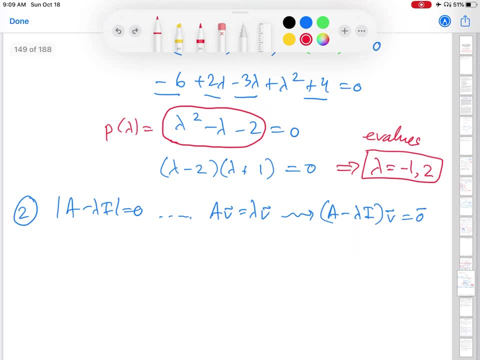 In this form. it's from there that then we then applied the first theorem in this lesson to give us this as a condition for the eigenvalues. Okay, so I'm going to go back to this form of the eigenvector eigenvalue equation And now this is what I'm going to use And in general, this is what you use to find the eigenvectors. I'm now going to substitute in the first eigenvalue into this equation and find the eigenvector, And I'll go back to the same thing for this eigenvector. 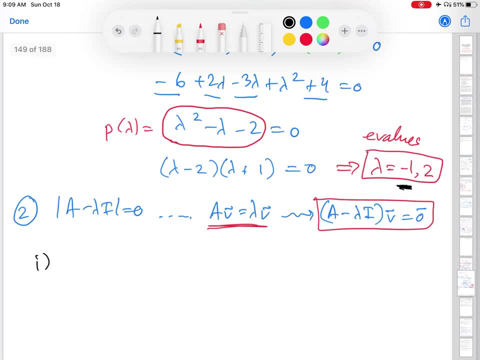 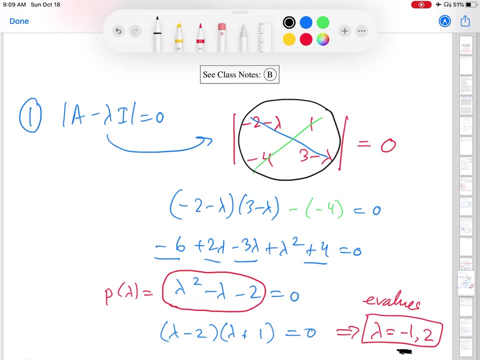 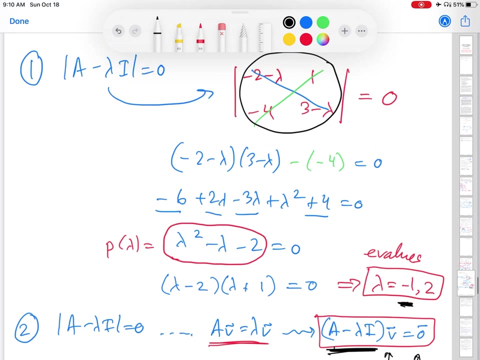 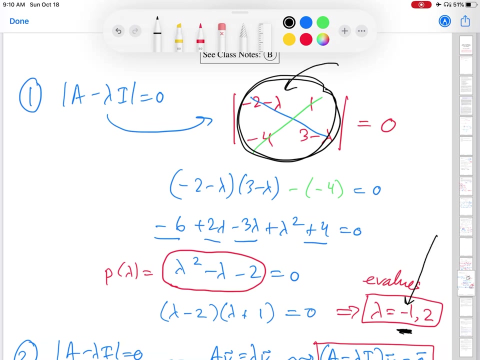 Okay, so the first thing I'll do here is: notice again: this is a minus lambda I. It's the same matrix that we found up here, except I'm not taking the determinant. Right now it's getting multiplied by v and set equal to zero. Okay, so a minus lambda I. So here it is. I'm going to plug in: lambda equals negative one for this in here and also in here. 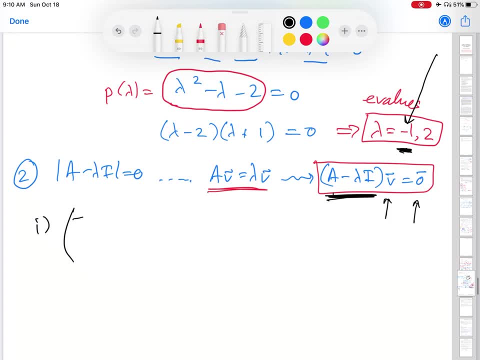 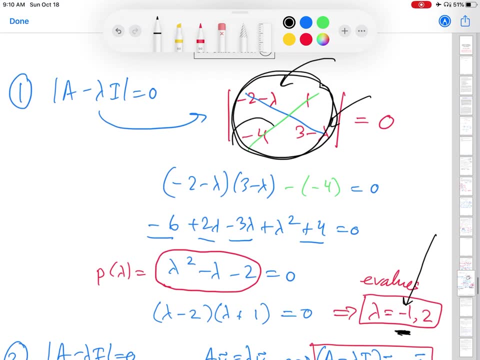 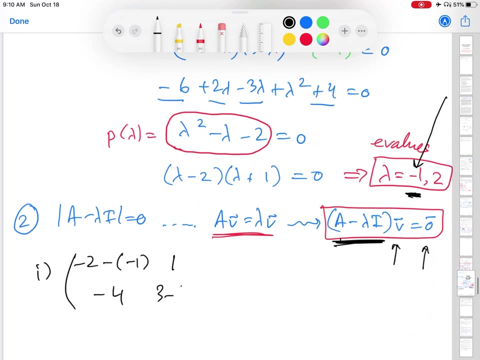 All right, so I do Negative two minus negative one, And then the upper right component is one, Then the lower left component up here, negative four, And then negative or three minus the lambda value, which is negative one. So I'm going to write this down here And now I'm solving this system, And the way I'm going to solve the system is using augmented matrices, Right, That makes it. 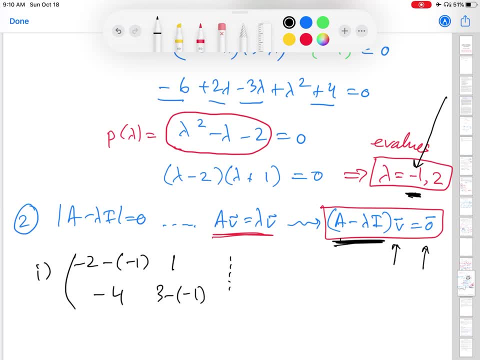 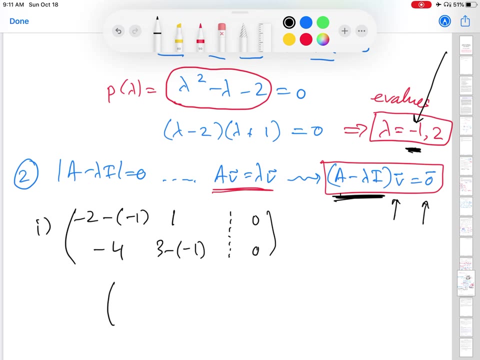 a little easier to get keep track of what's going on, And it also goes back to very, very early things that we had done in the first, really really the first lesson in this linear algebra unit. So to solve this, I'm going to simplify it a little bit. So I get negative two minus negative one, So negative two plus one negative one, And then down here I get three minus negative one, So I get three plus one four. 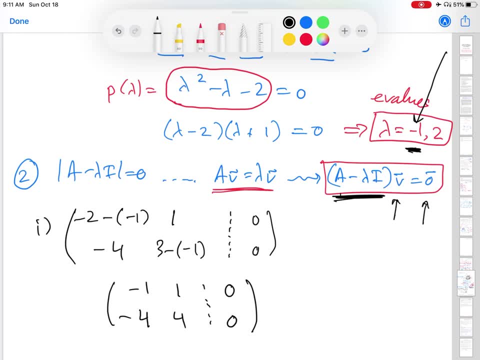 And notice: based off of all the things that we talked about in the in this lesson notes, we should get an infinite number of solutions, an infinite number of eigenvectors. So we are going to pick out one of those to form effectively the basis for the eigenspace, But we're going to pick out one of those as the eigenvector. So in this case, if I row reduce here, you can see that these two rows are exactly. 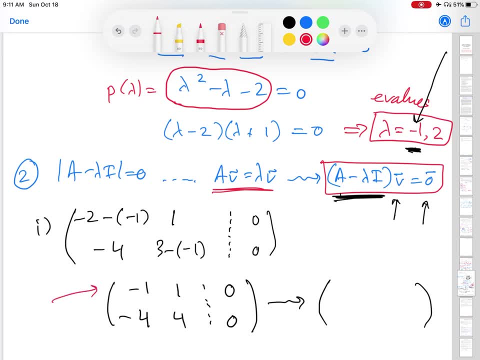 one of them is going to zero out, So I could keep the first row and then to zero out the second row. I could just multiply the first row by four and then add it to the second row, And that would give me all zeros. 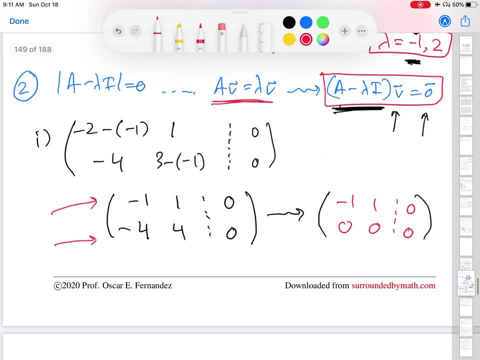 Okay, and I wouldn't have changed the first row, So I'll keep it that way. All right, If I now write this first equation, this first row, as an equation, The eigenvector V- here I'm going to say- has components V1, V2.. So this first row is minus V1, plus V2 equals zero, which tells me V1 equals V2.. 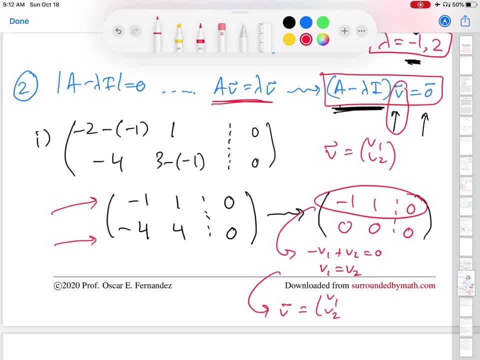 So my eigenvector V in this problem, which had to be zero, has components V1 and V2.. So this first row is minus V1, plus V2 equals zero, which tells me V1 equals V2.. components V1, V2, actually the two components are the same. So if I factor out the V1,, 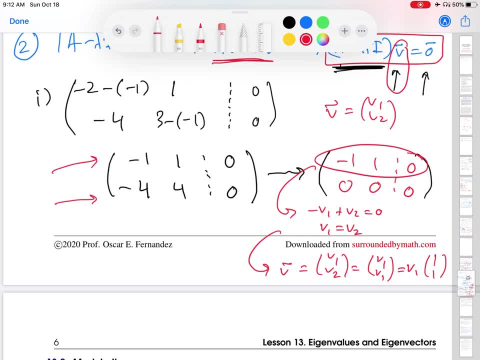 I get that And this is what I was saying, you know, just a minute ago. So all of the eigenvectors corresponding to the eigenvalue negative 1 that we've used are multiples of the vector 1, 1.. So we are going to call V sub lambda equals negative 1.. We're going 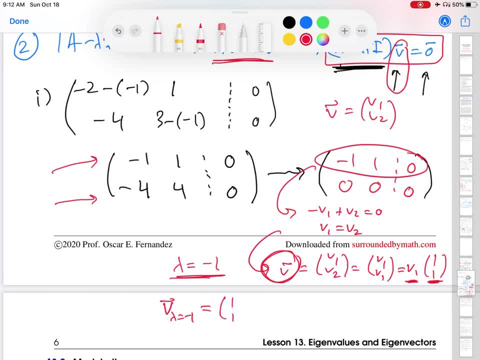 to call the eigenvector corresponding to this eigenvalue: 1, 1.. Okay, again, you could choose any other eigenvector, any other vector that's a multiple of 1, 1.. You could choose 3,, 3,, 7, 7, or something exotic like pi pi. right, It's totally up to you. But because 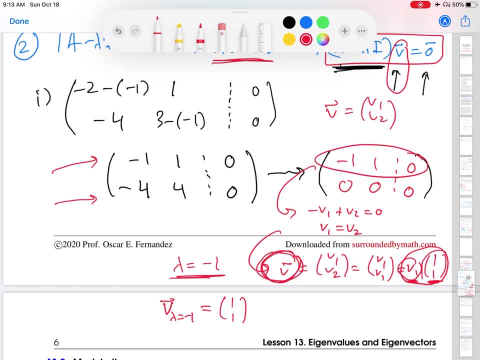 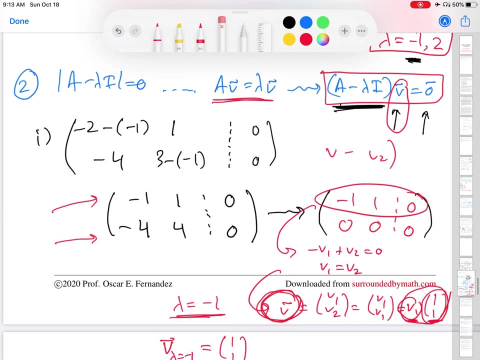 every single eigenvector is a multiple of 1, 1, and 1, 1 is a fairly simple vector, then that is the vector, the eigenvector that I'm going to choose for this eigenvalue. So what I'm going to do now is I'm going to erase all of this. You know I'm going to. 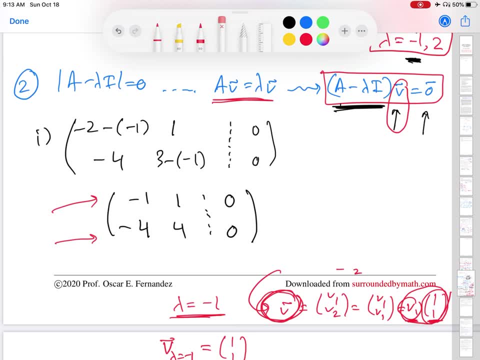 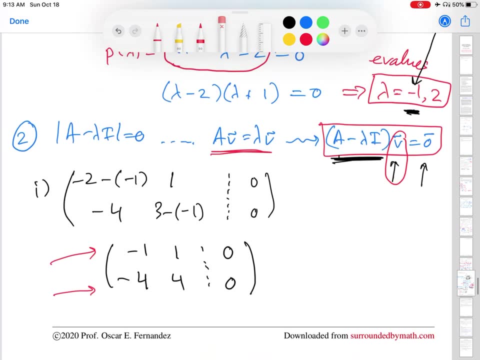 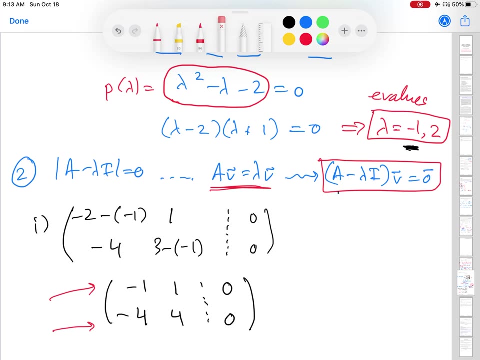 you know, just record up here that we found this eigenvector. Actually, I'll leave it down here And I'm going to go back, like I said earlier, excuse me and do everything all over again for the second eigenvalue. All right, so what's going to change is this: 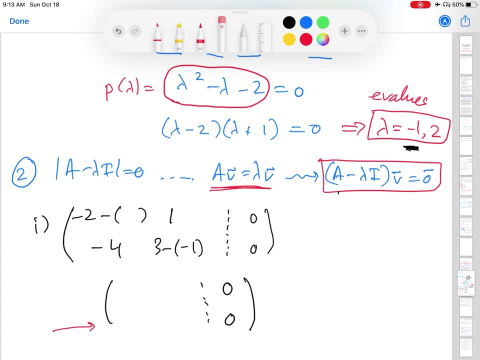 matrix and therefore the row operations And therefore the eigenvector. So let's go back and redo this calculation, for the eigenvalue of lambda equals 2.. So I'm going to put it here right, And then I'm going to redo the. 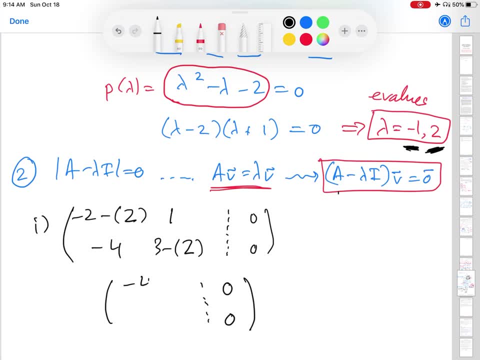 arithmetic. So now I have negative 2 minus 2, that's negative 4.. Keep my 1, negative 4.. And then 3 minus 2, that's 1.. And so again you know, you can zero out the. 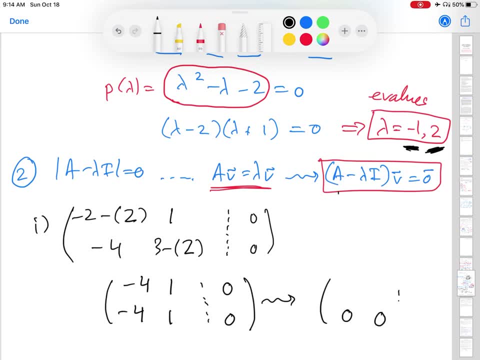 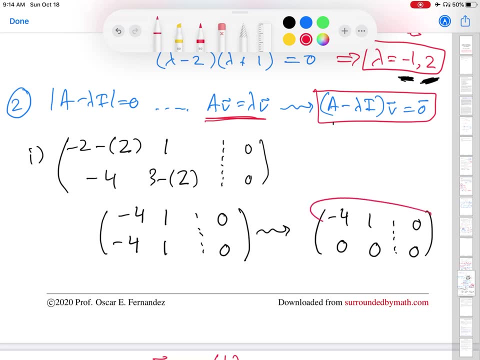 second row by just multiplying the first row by negative 1, and then adding it to the second row, And that leaves this first row. So if I take this row and write it back out as a system, minus 4v1 plus v2 equals 0.. I will confess I have a little bias against.